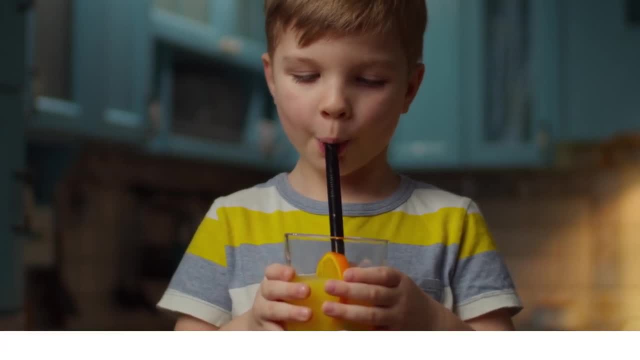 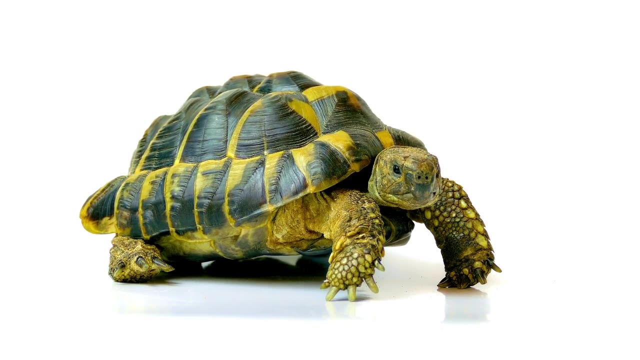 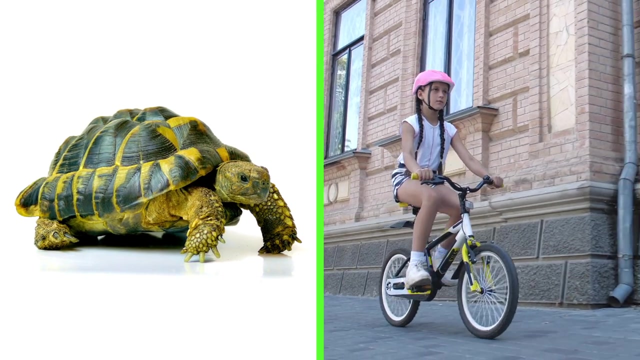 Humans invented drinking straws that work the same way. One special body part of a turtle is its shell. A turtle's shell is very hard. It protects the turtle's body. Humans copied the idea of a turtle's shell to create helmets. A helmet protects a person's. 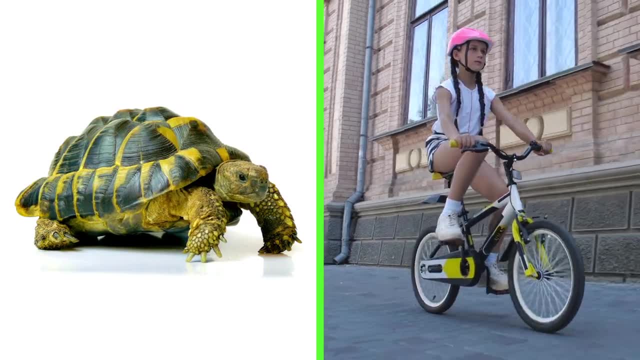 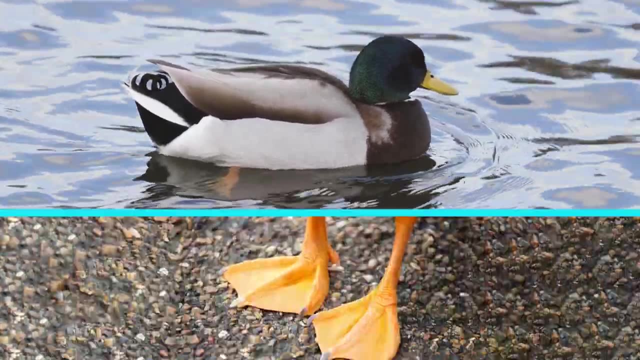 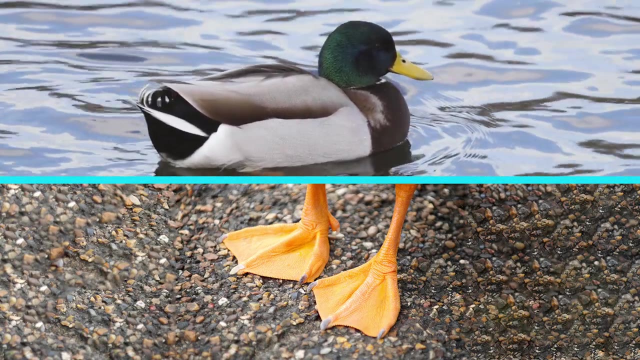 head, just like a turtle shell protects a turtle. Here is a duck. What part of the duck inspired a human invention? Ducks have webbed feet. This means their toes are connected by skin. These webbed feet help ducks paddle through the water. 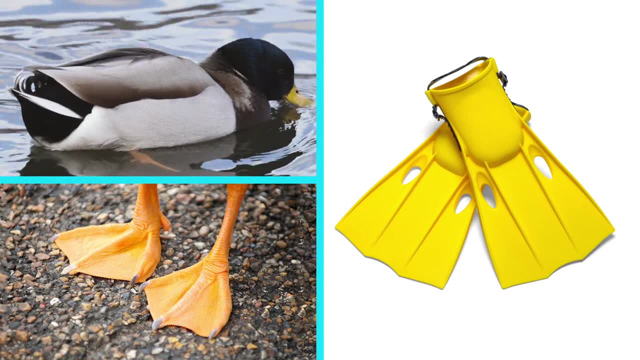 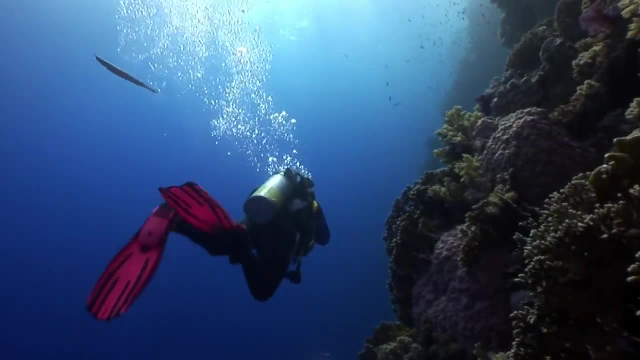 Humans designed an invention called swim fins or flippers. A swim fin has a shape like a duck's foot. People wear swim fins to move more easily through water while scuba diving or snorkeling, But in the past, humans have used a swim fin to transport the water to the ocean. 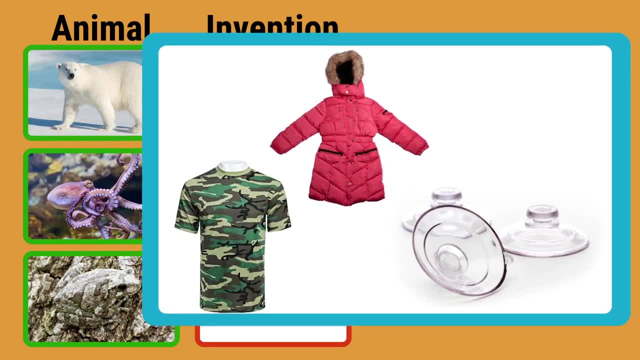 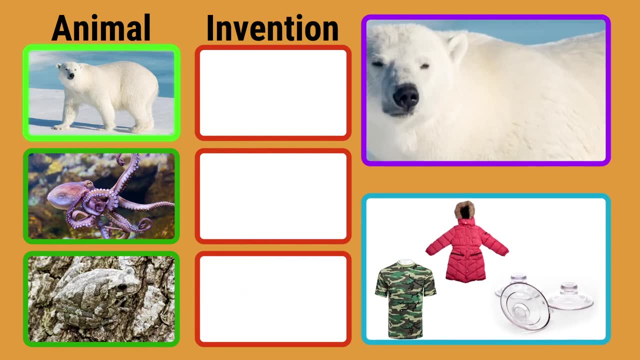 Here are a few more inventions in the world of swimming inspired by animals. Can you match each animal to the invention it inspired? Take a closer look at the polar bear. It has very thick fur. This fur keeps the polar bear warm in the freezing Arctic. People do not have thick fur like a polar bear. Instead, humans took the idea. 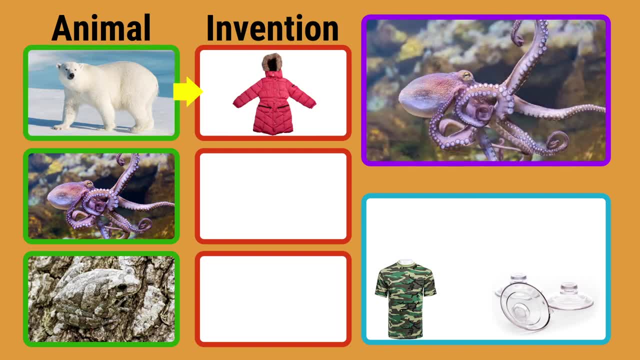 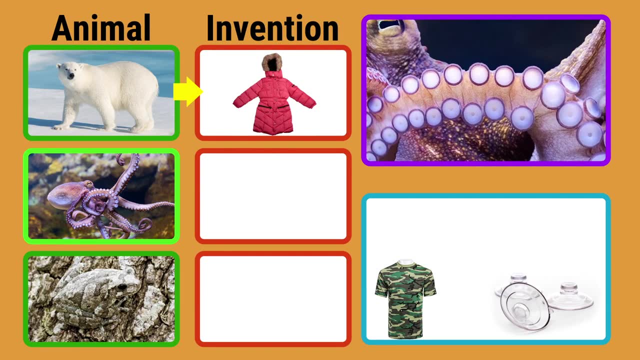 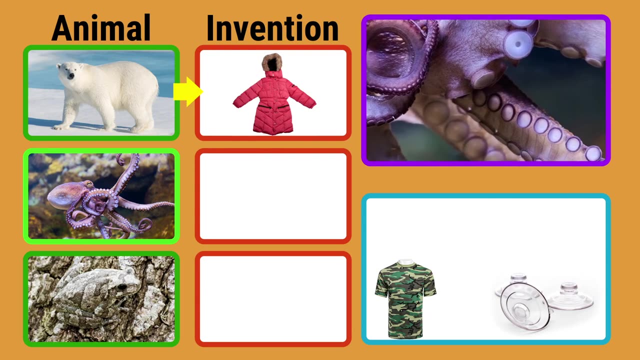 and designed coats to wear in cold weather. What about the octopus? What part of this animal did humans copy? Do you see the round things on its tentacles or arms? Those rings are called suckers. Octopuses use suckers to touch and taste. Suckers are very useful for holding. 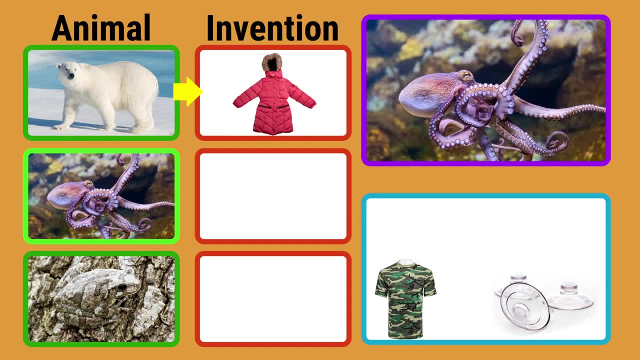 onto things too. This body part inspired people to design suction cups. Suction cups work just like an octopus's suckers: When they are pressed to a surface, they cling to it. Suction cups can be used to press a surface. These are used to press a surface to a surface. 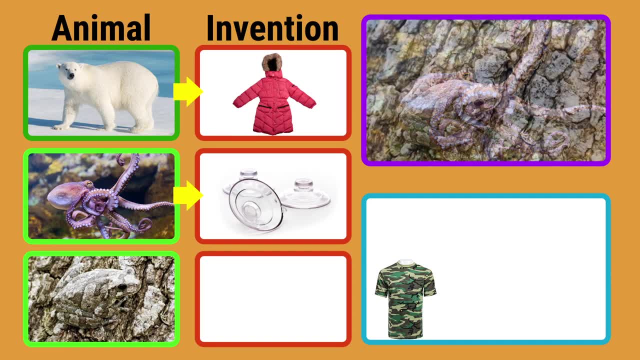 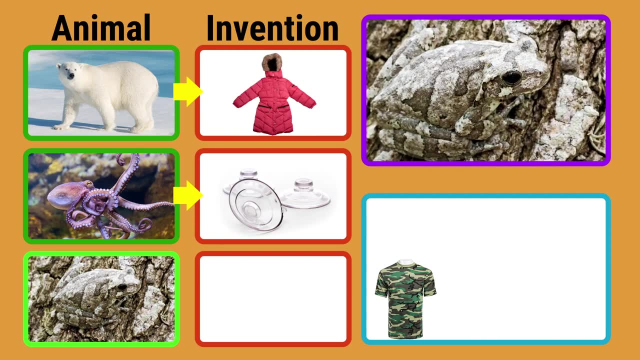 Suction cups are used to press a surface. These are used to press a surface. These are used to Caution cups have many uses. There is one more animal. Do you see it There in the tree? it's a frog. The frog is difficult to see because the color and pattern of its skin match the tree bark.